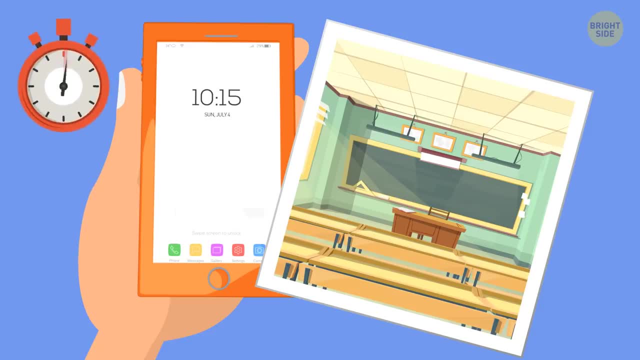 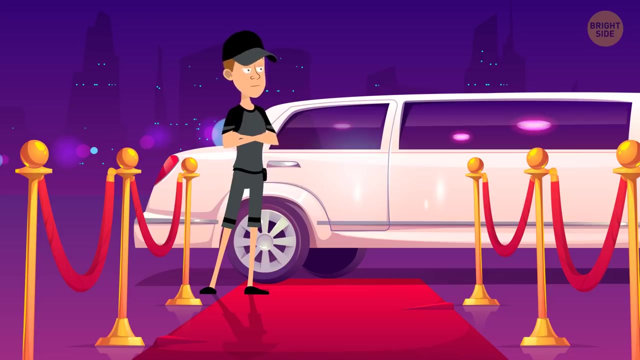 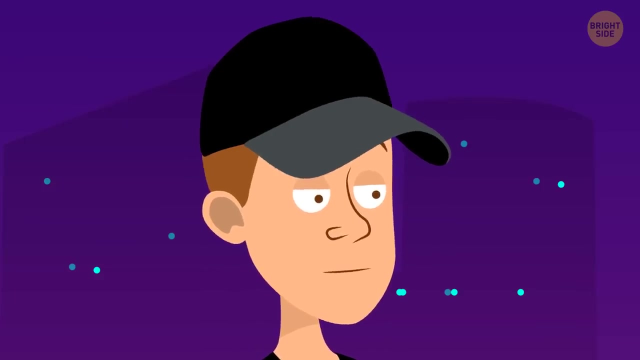 How did she understand Eveline wasn't at school? Look closely at her cell phone. It's Sunday. There's no school on Sundays. Ned works in a club. His job is to check people's ID cards and to not let suspicious people or people younger than 21 years old get inside. 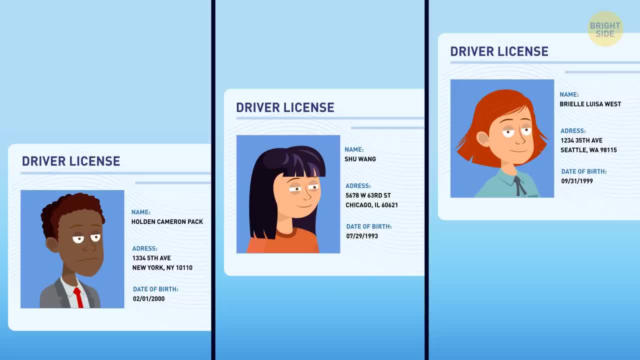 Take a look at these three ID cards and figure out who shouldn't enter the club. The first person is already 21, and nothing else looks suspicious in his ID. The second girl seems all right too. It's written that Brielle was born on Sunday. 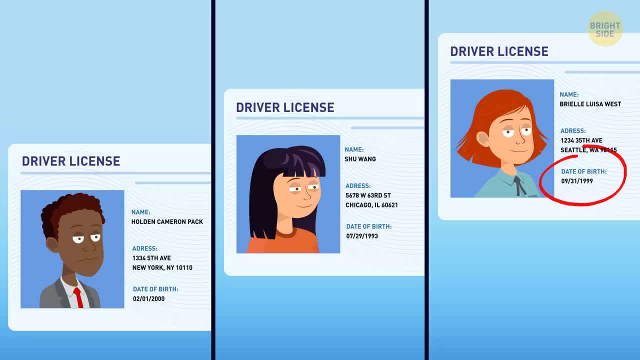 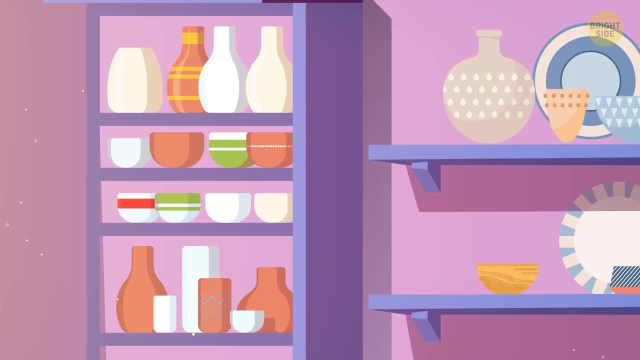 She was born on September 31st, Ah, but such date doesn't exist. Her ID must be fake. Mrs Cabell is the owner of a small company producing expensive designer cups. On Friday, when the working week was finally over, 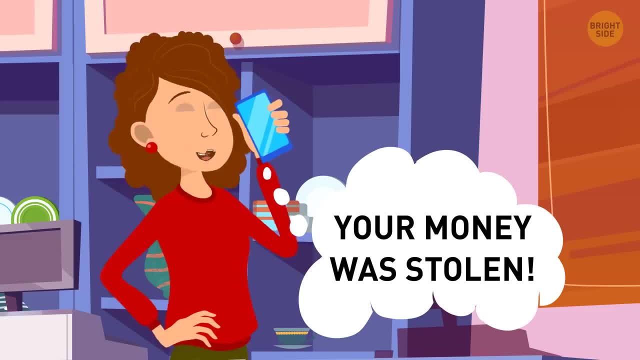 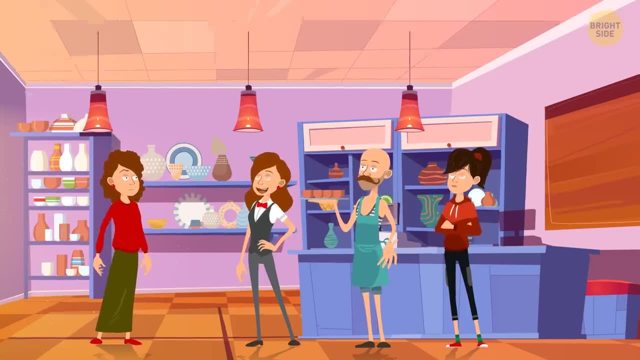 she got a call from her bank. The woman found out that someone had stolen all the money she had saved. Mrs Cabell realized it must have been one of her workers, so she asked each of them what they had been doing that day. 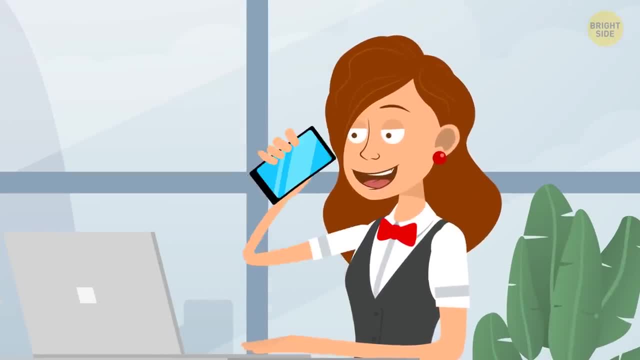 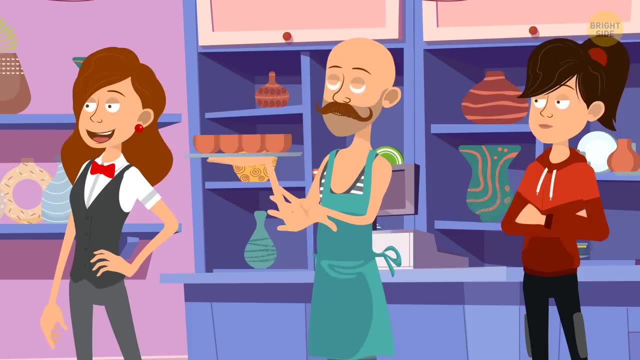 Sloan, a sales manager, said she had been talking to their clients and looking for new ones. Atticus, a potter, said he always made one cup a day and he showed all the cups he had done that week. Sierra, a designer. 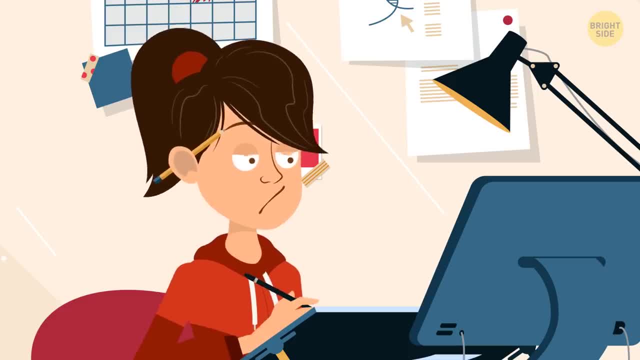 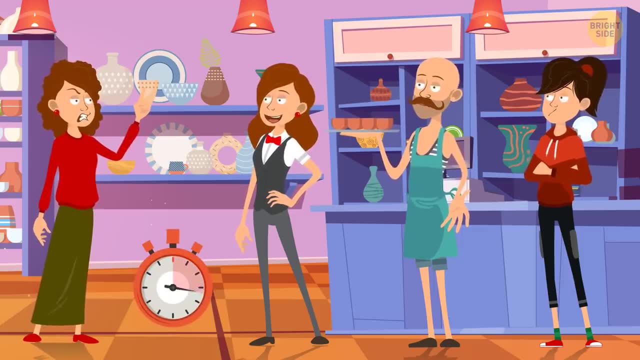 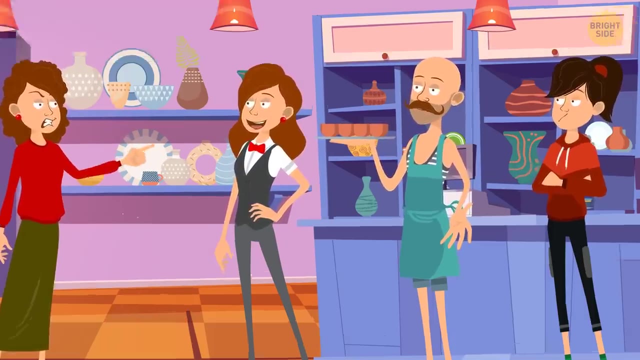 said she had been working, but she also admitted she hadn't been really productive that day because of some family issues. Who lied, Atticus? There are five working days in a regular week. The man said he made one mug a day, but he only showed four mugs. 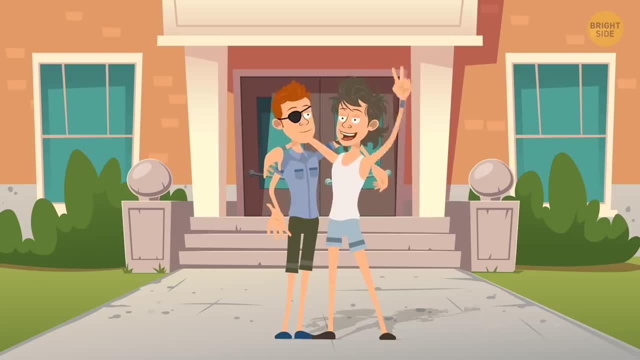 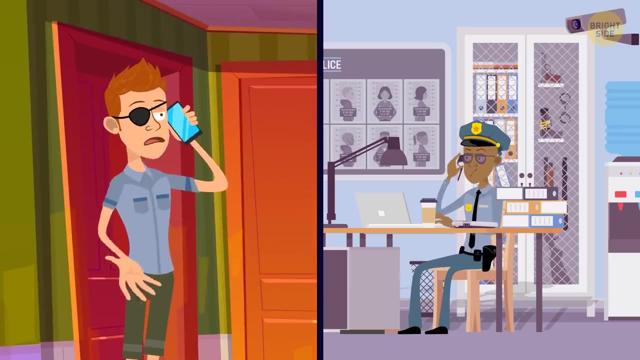 It means he missed one day of work. Lennox and Finn were friends living in the same college dorm. One day Lennox reported that something had happened to his friend. He said Finn hadn't left his room all day. He also never responded to any of Lennox's texts. 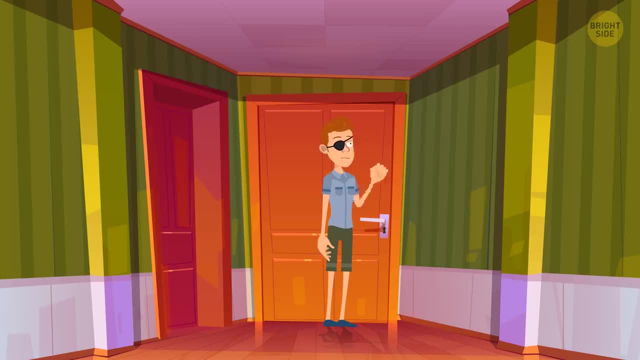 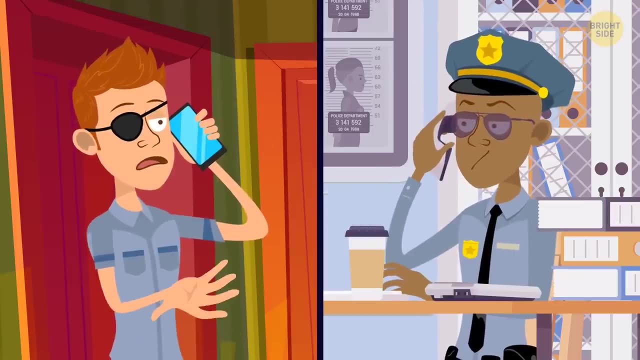 In the evening Lennox started to worry and knocked on Finn's door, but the guy didn't answer. Lennox peeked through the keyhole and saw that his friend was lying on the floor, So he called the police. After that, Lennox got arrested. 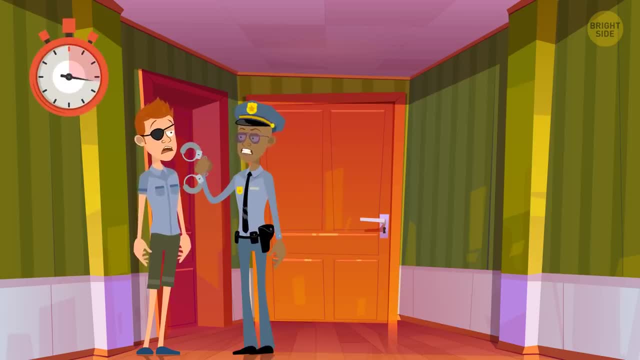 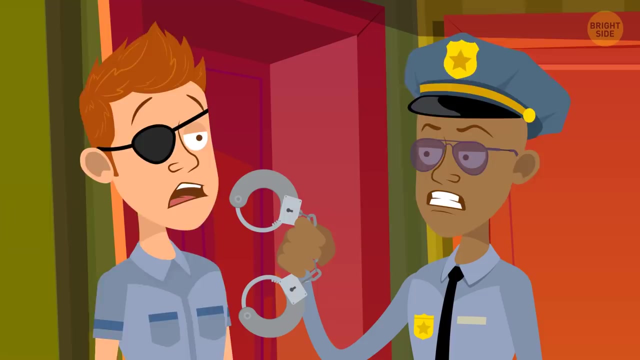 Why Lennox has a bandage on his right eye, but the keyhole is located in such a way that it's only possible to look inside with the right eye. It means the guy couldn't do it. He simply knew what had happened. 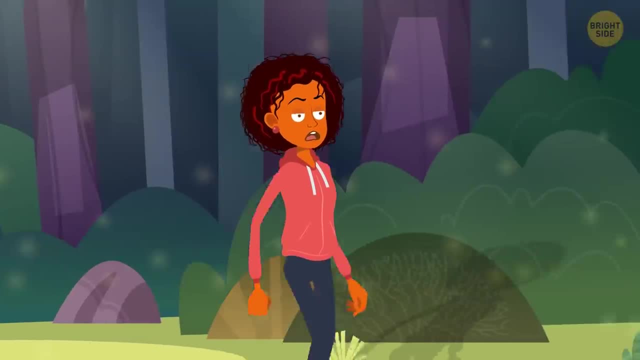 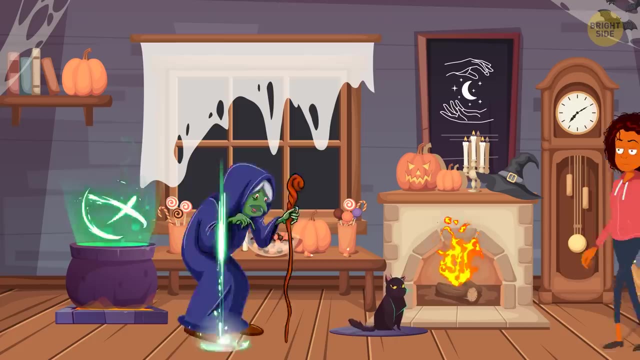 Esme was having a walk in the forest and got lost For about the 20th time. Hey, don't ask. Anyway, she found the witch's house, walked in, said hi, petted the cat and asked the witch to show her the way home. 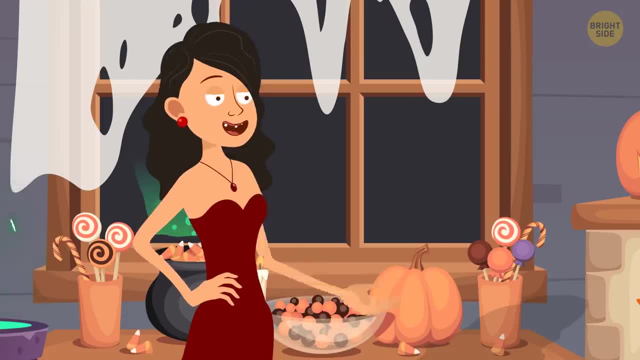 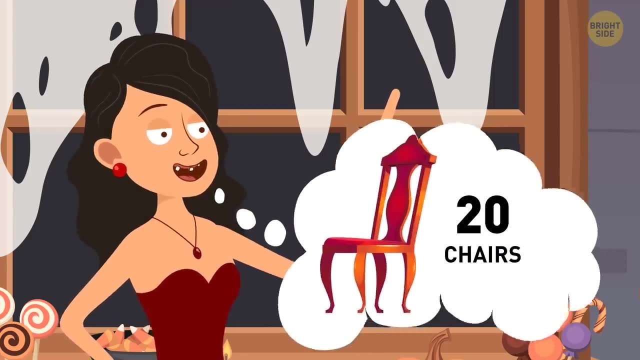 But the witch had a problem. She was learning a new spell and accidentally did something strange to her chairs On the bright side. she now had a riddle for Esme to solve. The witch had 20 chairs. Now some of the chairs only had two legs. 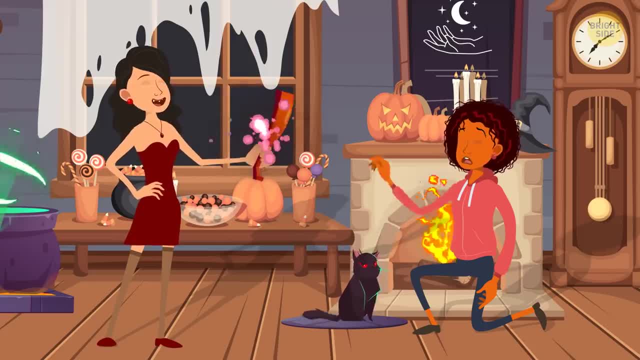 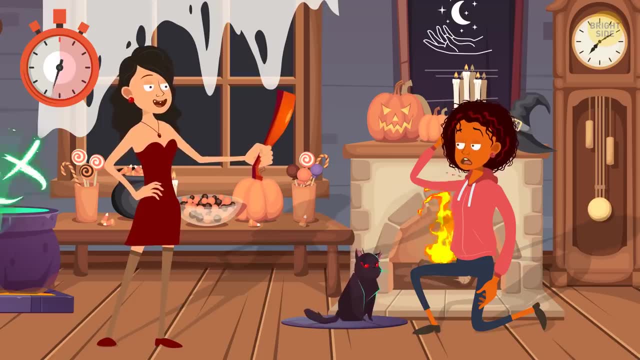 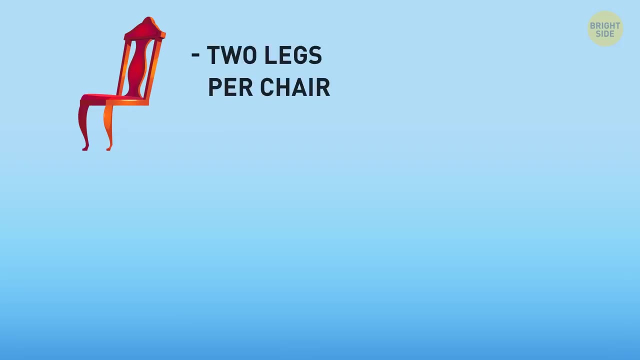 and half of the rest had no legs at all. How many legs did all these 20 chairs have in total? We know that some of the chairs have, on average, two legs per chair. The rest of them have either four legs or no legs at all. 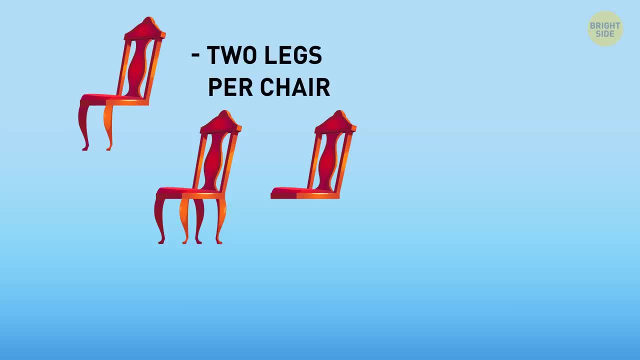 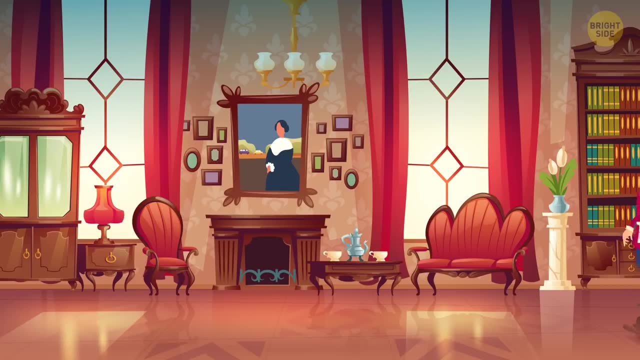 And since half of the rest have no legs and the other half have four, together they have two legs per chair, So there are exactly 40 legs. Mr Tucker was a businessman. He was a businessman. He wanted to find an interesting hobby. 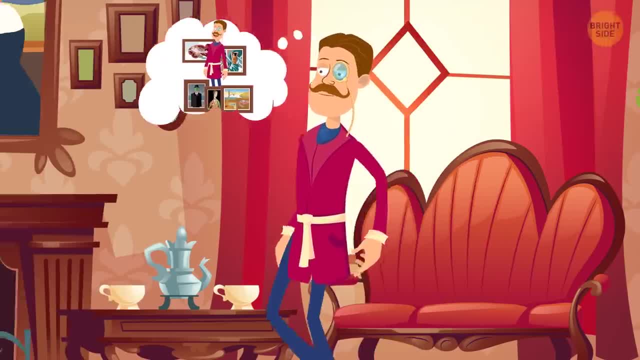 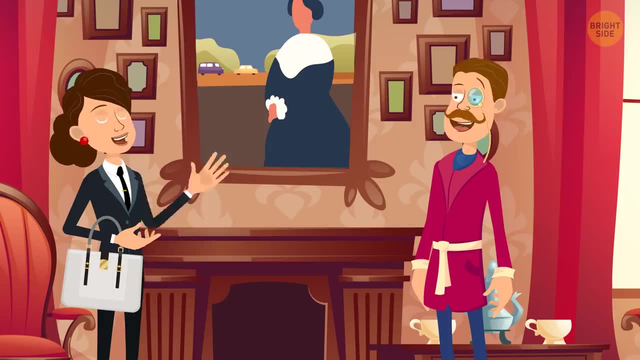 to impress people. He chose art, even though he knew nothing about it. Still, he kept buying paintings and even owned a couple of famous masterpieces. He liked to invite his potential business partners over to show off his collection One day. his guest was Miss Geneva Darby. 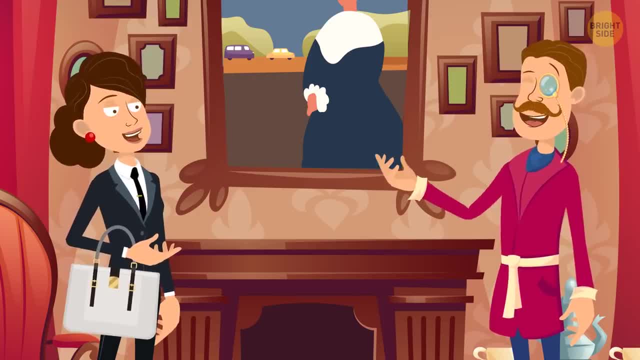 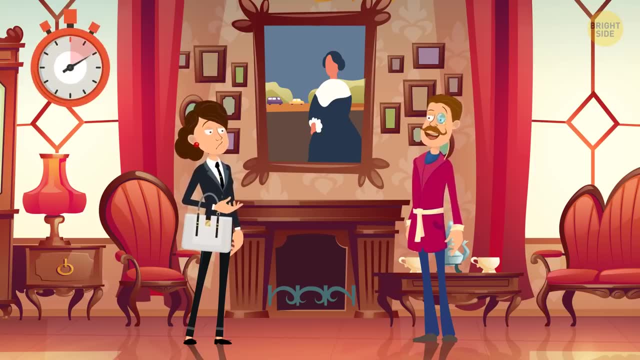 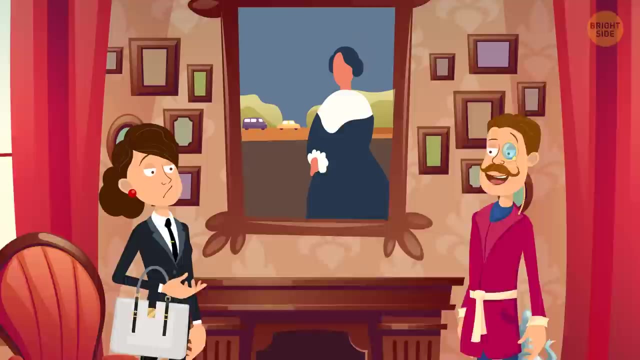 a young lady who owned a jewelry business. As always, Mr Tucker boasted about his collection, But Miss Darby wasn't impressed. Why Look closer at this supposedly 16th-century painting? There are a couple of cars on the road. 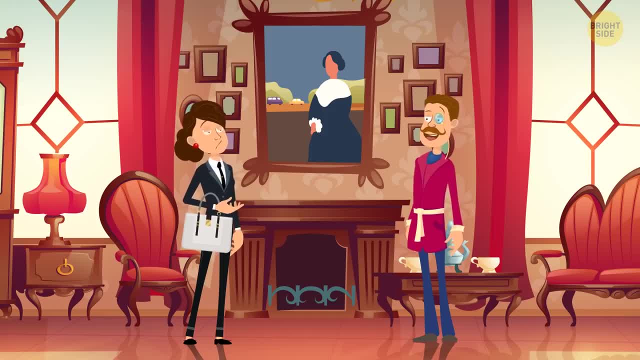 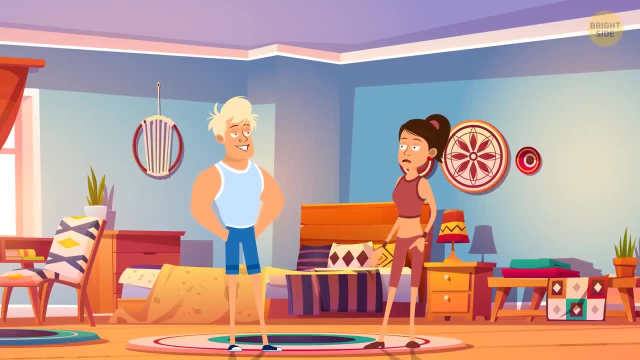 But there were no cars at that time, so the painting must be fake. Evie and Kai were planning to go on a bike tour with their friends. Unfortunately, Evie didn't feel well, so she canceled on her friends and asked Kai to stay with her. 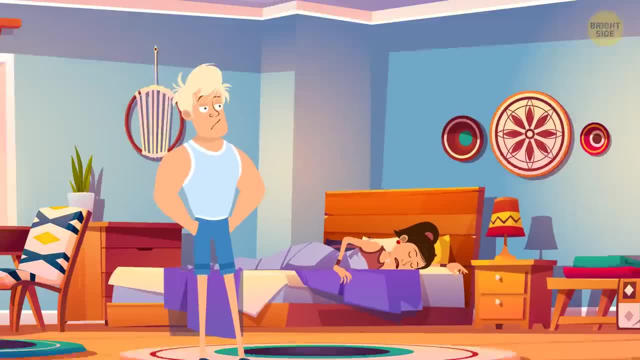 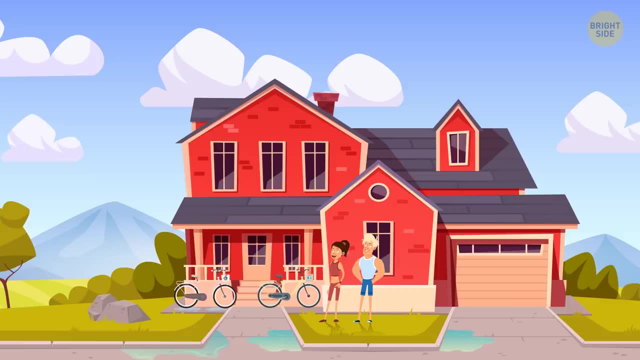 Kai was disappointed but agreed. Evie fell asleep. When she woke up she already felt better. She offered Kai to ride their bikes a bit, just the two of them. But when they went outside, Evie realized that while she had been sleeping, 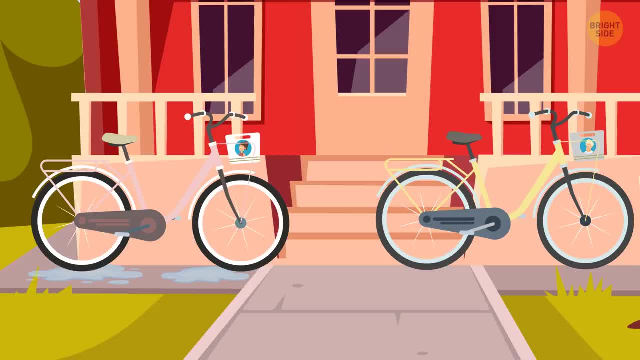 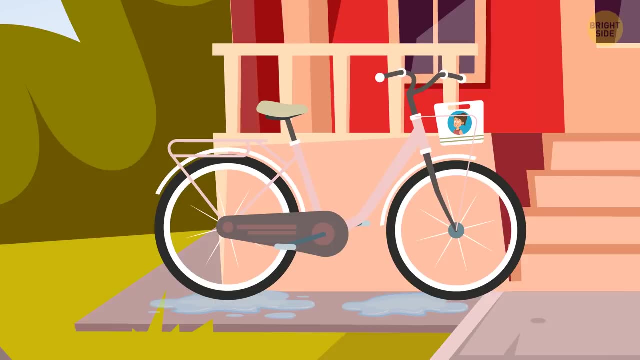 Kai had been out with the friends without her. How did she understand it? Look, Evie's bike is all wet. It must have been raining while she was asleep, But Kai's bike is dry. It means that he used it and then wiped it off. 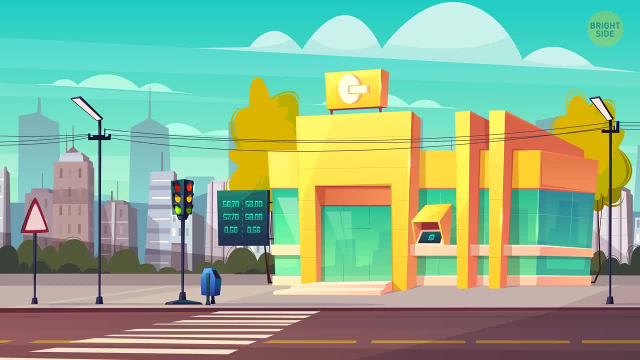 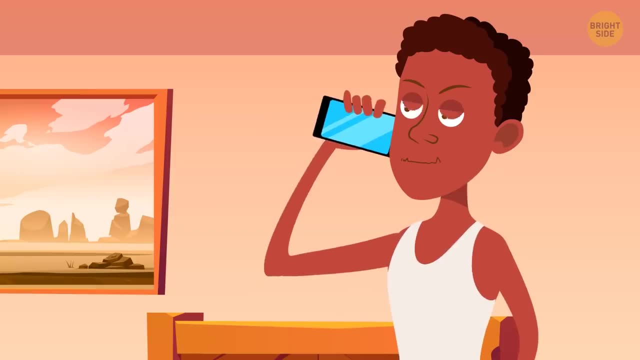 Or maybe he wasn't even in the area when it was raining. Two weeks ago a bank was robbed But the robber hadn't been found yet. A phone call woke Detective Callum up in the middle of the night. His colleague reported that a farmer had found the money. 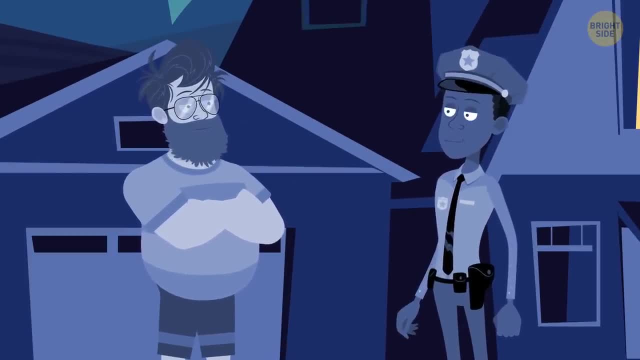 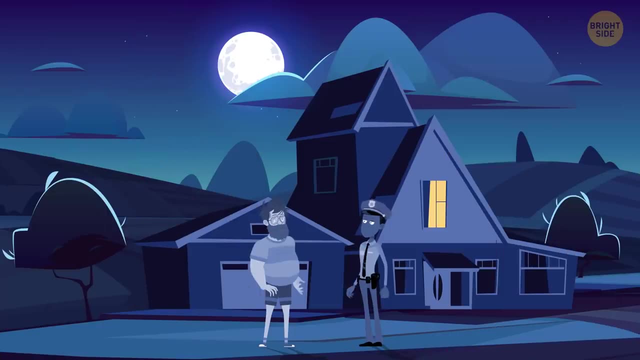 When the detective arrived he questioned the farmer. The man said I argued with my wife and went outside. That's when I found a bag with money in a cornfield. Detective Callum asked if the farmer's wife was there. He said 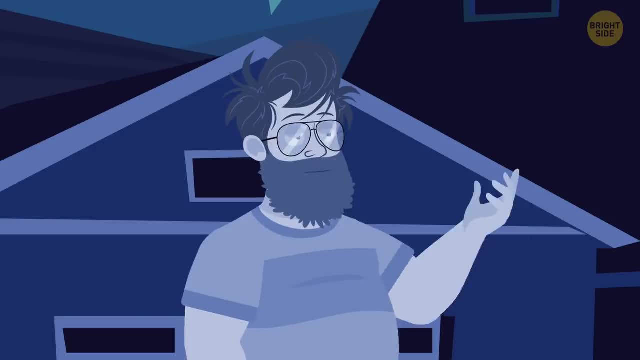 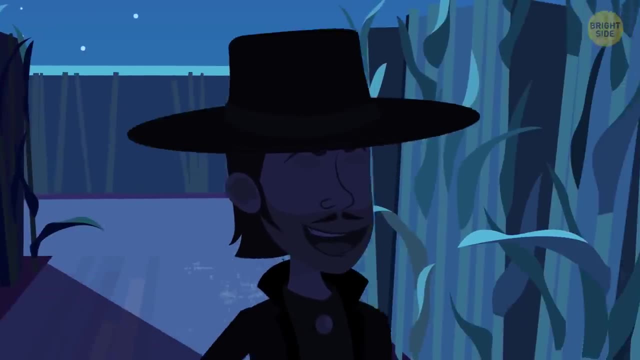 He said. He said The farmer had noticed anything suspicious before The farmer replied. About two weeks ago, before going to bed, I looked out of the window. I saw a man walking through the field. It was a full moon and I could clearly see his silhouette. 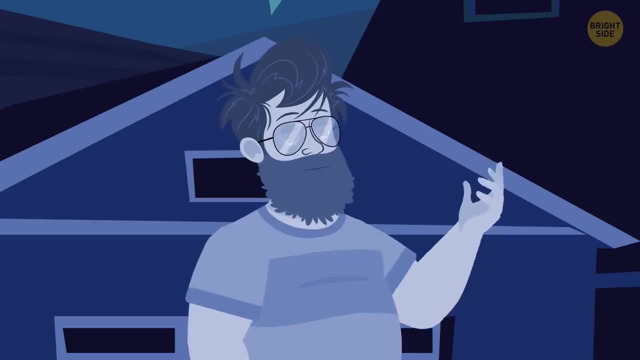 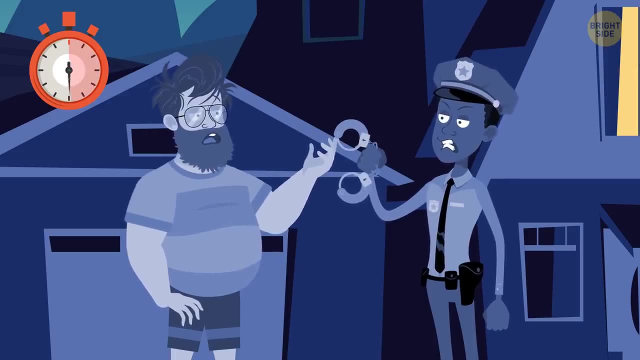 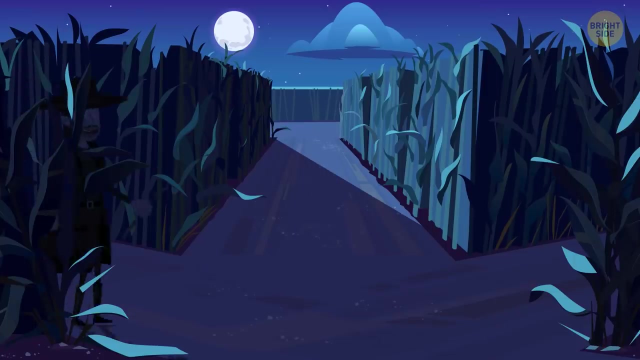 But there wasn't enough light to notice more details about him. The farmer was arrested, Why? The farmer said it had been a full moon two weeks before, But it's impossible. As you see, it's a full moon now. The farmer is lying. 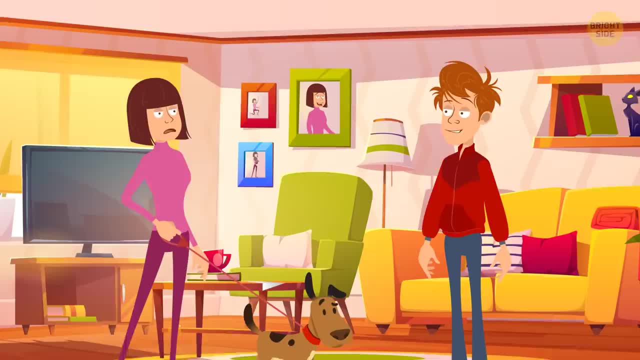 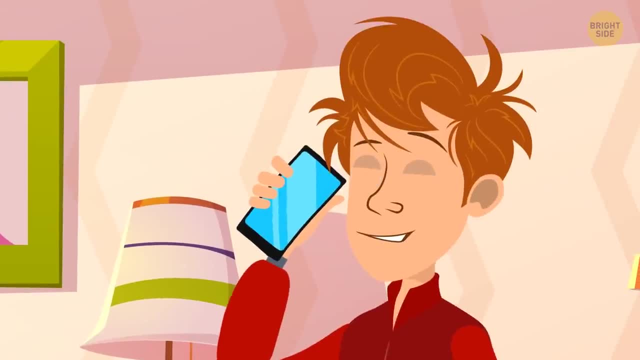 But why. Ashley was hurrying to an unplanned business meeting. She asked her boyfriend, Dean, to walk the dog. Dean agreed, But then his friend called and invited him to play a new video. So the guy decided to skip walking the dog that day and joined his friends. 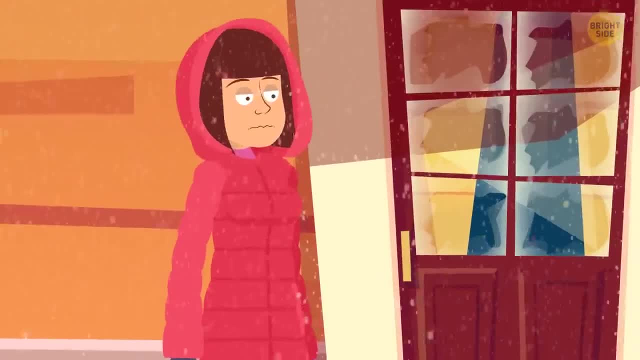 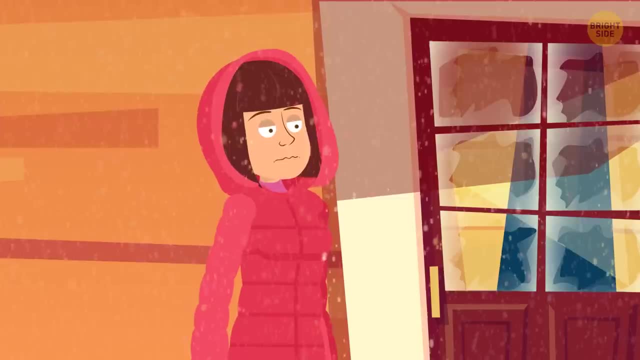 He and Ashley met right outside the house when they both were going back home. Ashley asked what Dean had been doing. The guy said I walked the dog and then went to play video games with my friends. Ashley immediately understood he was lying. How did she figure it out?